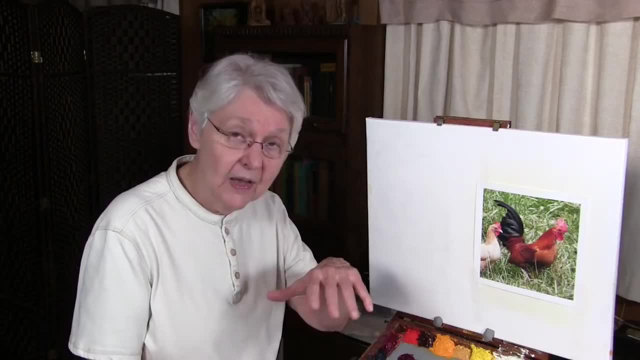 where the light is in shadow. So if you can build that skill first, you're halfway there, because if the area is in shadow, then it's in a very narrow value range. So if you begin there, the light is being blocked. Let me say it that way. So you can always do that. but let's just 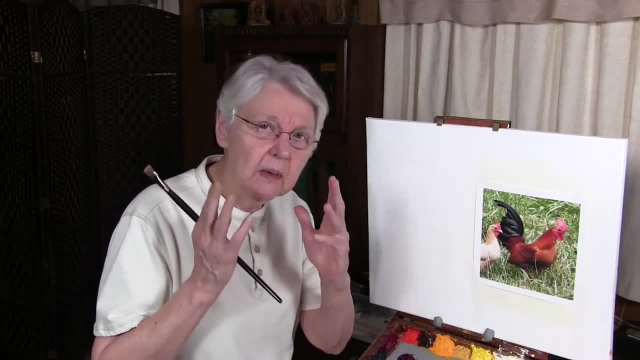 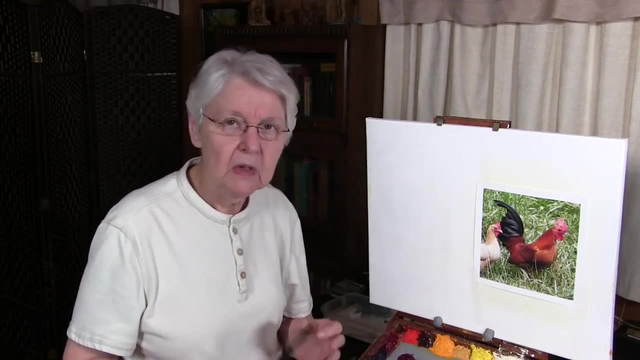 start right there with that one premise. If you can determine what's in shadow, All right. from that point, what is the darkest value you see? Now, as I said, this is going to be comparative. So what is the darkest value you've seen? If I'm looking at these chickens which we've used in a 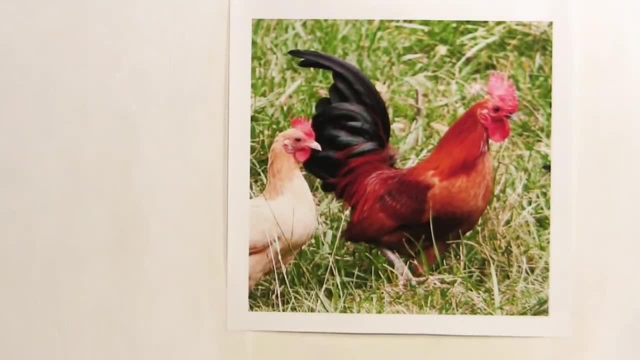 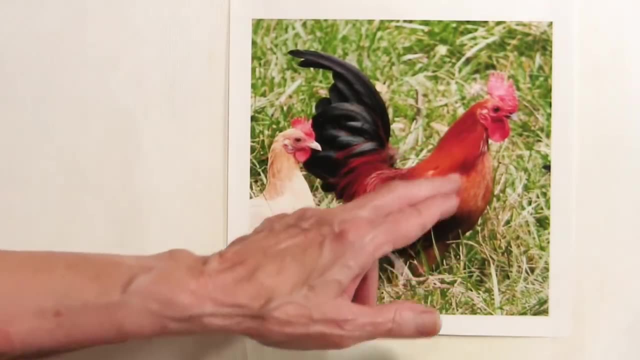 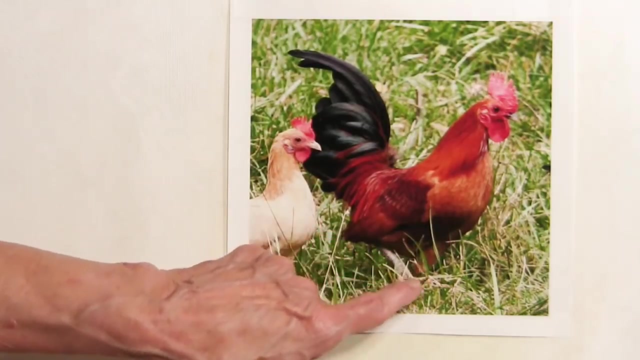 previous quick tip, or this rooster or whatever, what is the darkest value I see? And so he said: read color values. Well, even if I were looking at just this part of that rooster, what is the darkest value I see? Well, the darkest value I see is this value, right here. 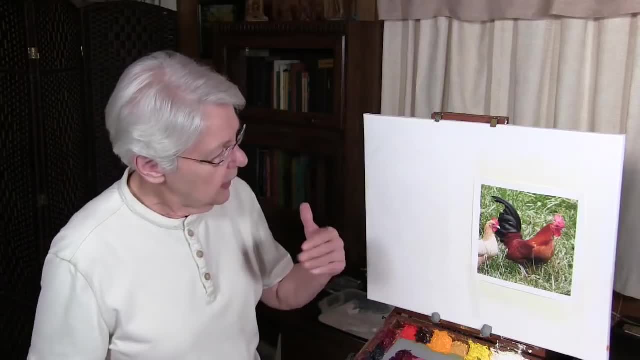 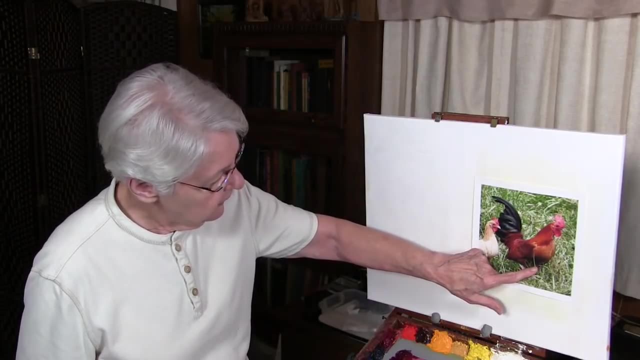 and you can see that is in shadow. Then I could ask myself: what is the lightest value I see? Well, let's start here first. What is the darkest value I see And can I match that value? Now, one really good system for doing that, for matching value. 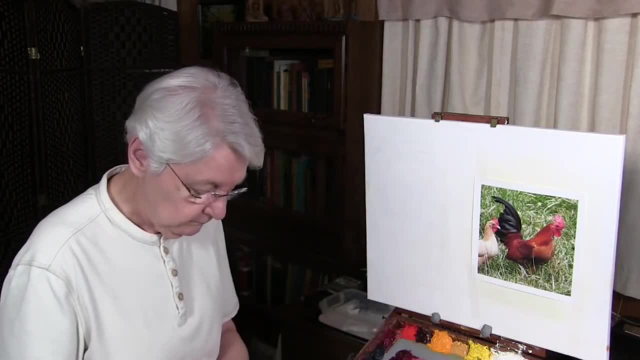 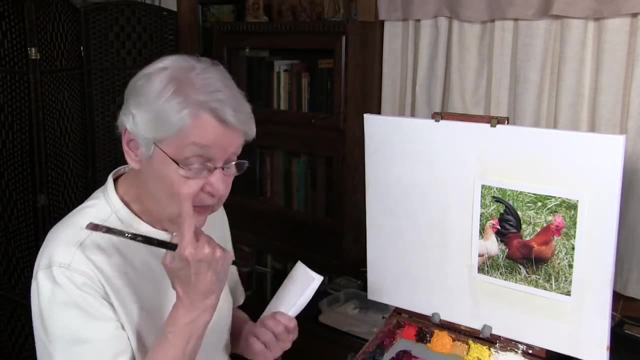 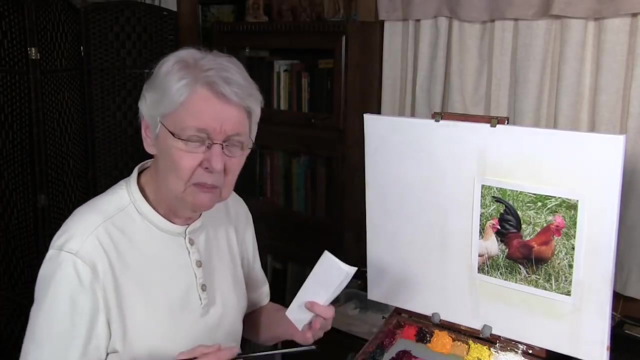 is. you can just take simple sheets of paper and you can do it this way. You say, okay, what is the darkest value? I see right here I can tell it's very dark. Maybe it's not the darkest dark that exists. Maybe this, even this would be black, would be the darkest dark that exists. perhaps. 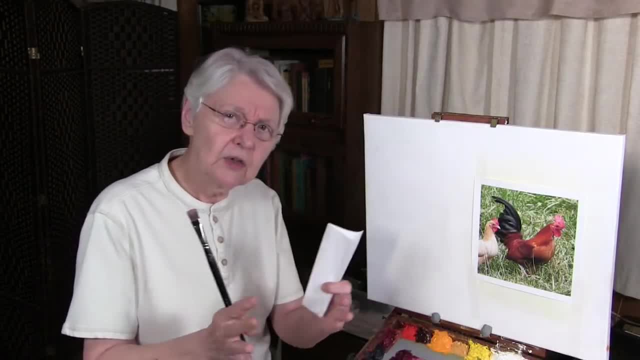 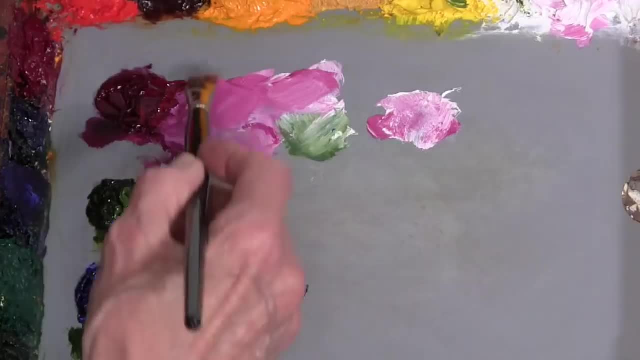 But it's a little lighter than that. So now you're using a little bit of comparative language and from that point you would begin to, you begin to mix towards that value. So now let's see, I say it's a little bit lighter than. 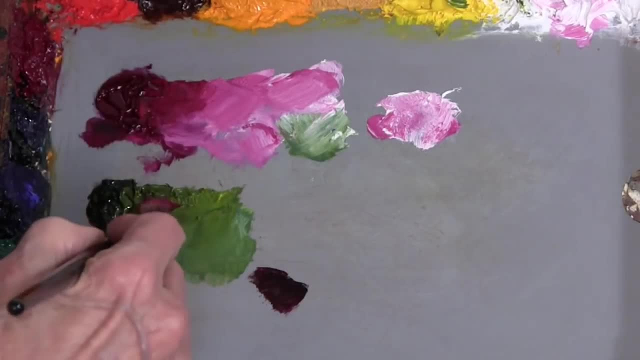 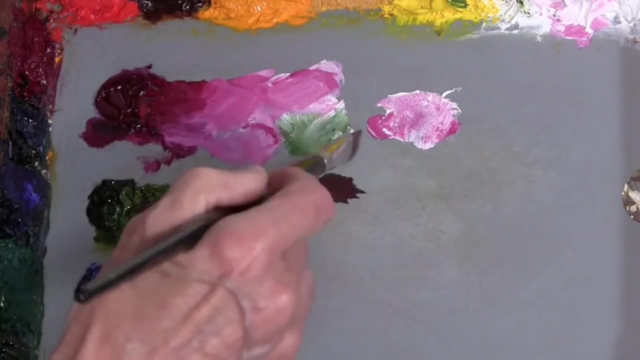 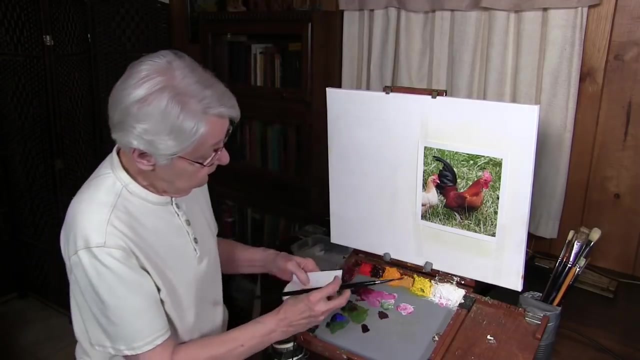 black. So if- and I see that that's sort of in a reddish, reddish green, and the viewer didn't ask about mixing colors, just about mixing the values, And so you could whatever you read the color to be, then let's put this just a little bit more like this. Then, if you put a little 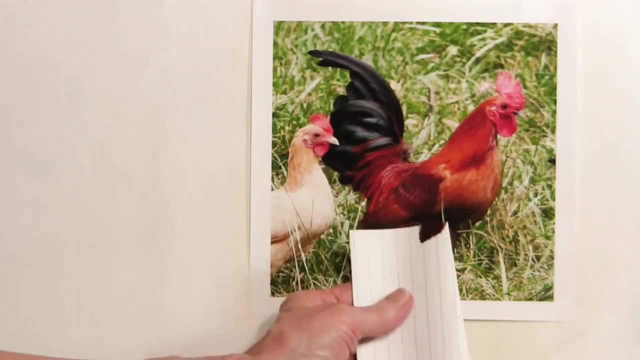 sample right here and you put a little sample right here and you put a little sample right here. hold it up to here. close one eye Now, if I hold that up, and I just say they seem to be in the. 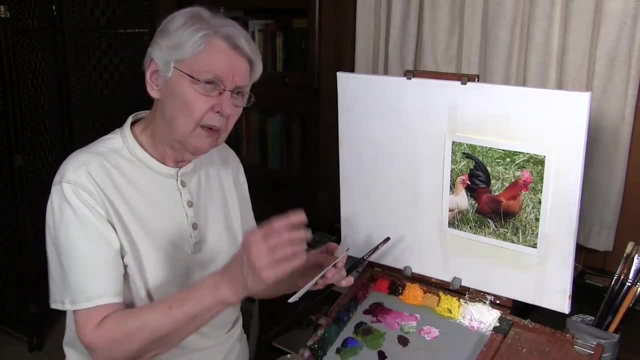 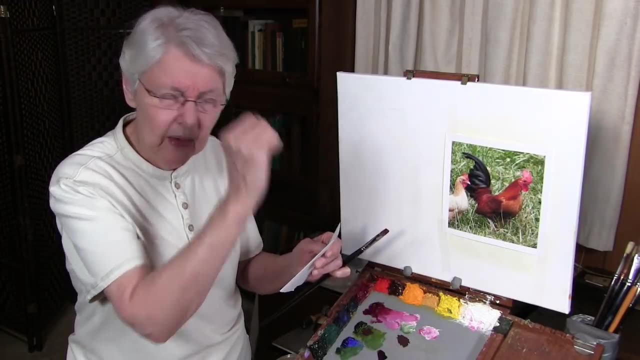 same value. I can do the same thing out in the real world. If I spot a value and I'm and say I'm not quite sure what I'm looking at, I can isolate that value, I can mix, just begin mixing. 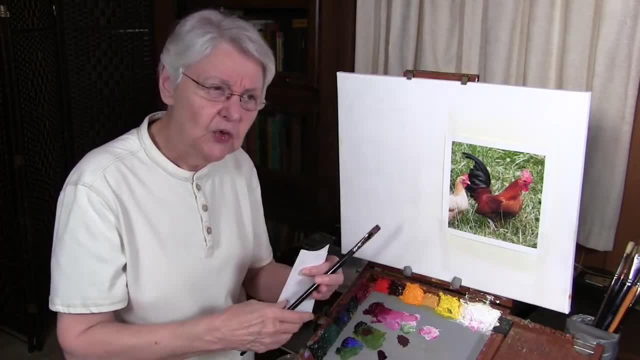 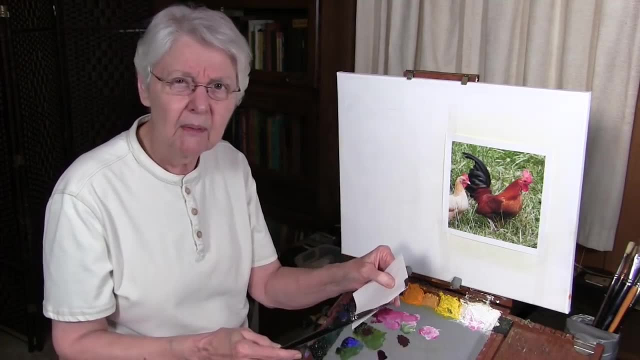 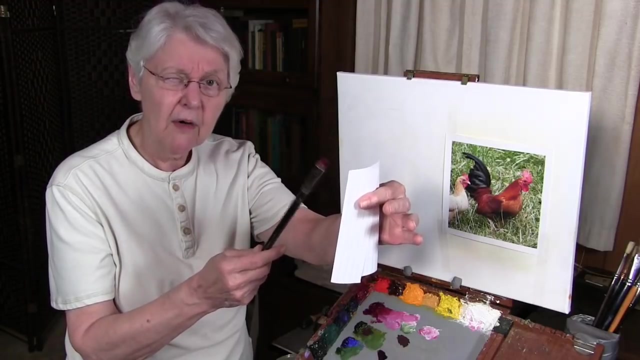 anything and then ask yourself what you need to add to it. Make a little bit of a sampling on the edge, right on the edge of a piece of paper, Anything. Hold it up close one eye, compare: Is my paint darker than what I'm looking at, or is it? 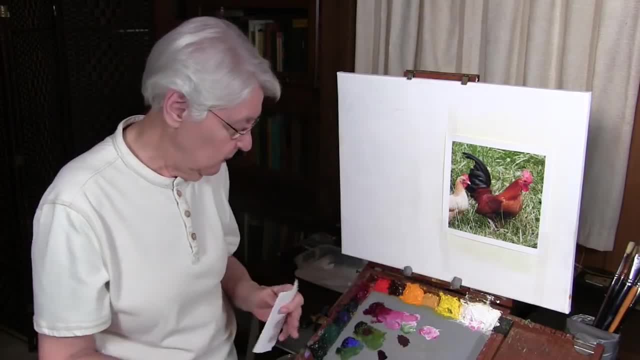 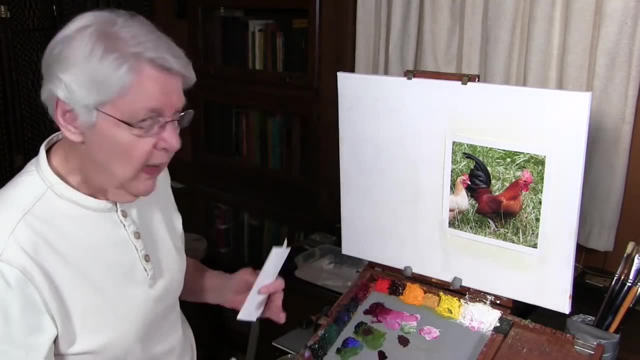 lighter than what I'm looking at. If it's darker, that means I need to add more dark. If it's lighter, that means I need to add more light. So that's one of the best ways to read that. Now, another way to: 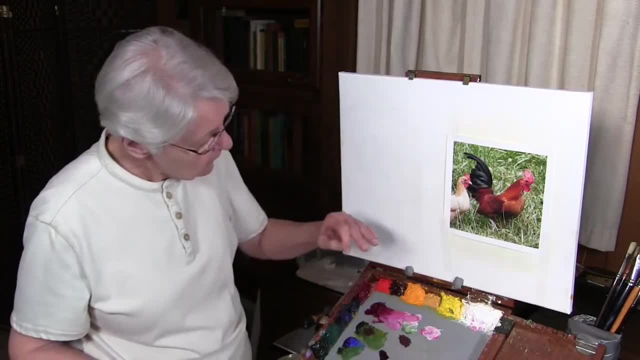 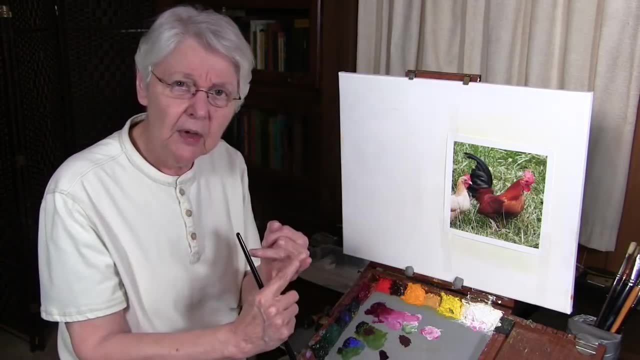 think about the whole issue of value is to compare The thing that you're looking at if it's the rooster, compare the darkest value you're looking at to the lightest value you're looking at. So, if this is the darkest value- and I'm just going to put this- 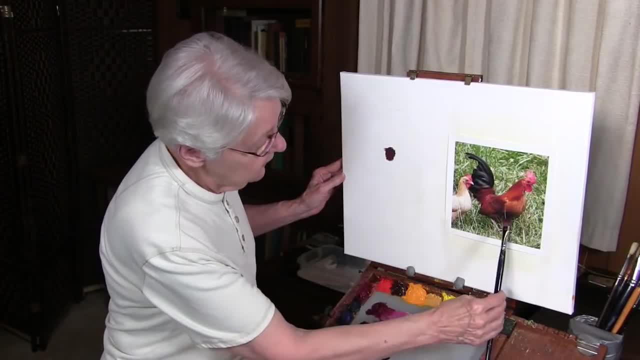 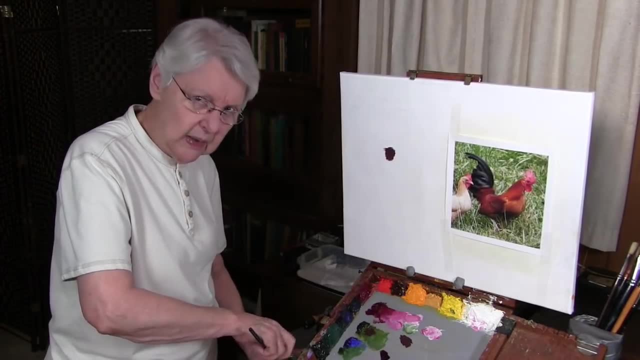 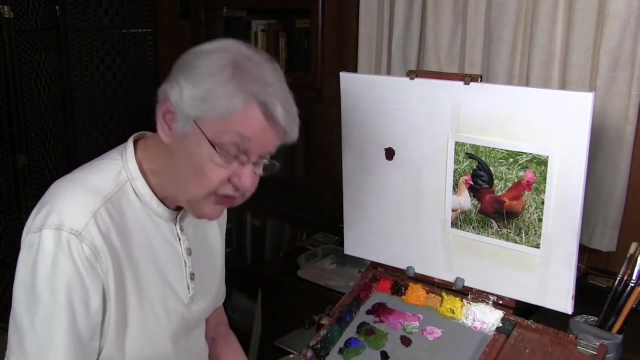 right here just as a value splotch, now that we have discovered that that is. that is pretty much the same value as that darkest dark I'm looking at. So you're not looking at color here, necessarily. Well, you're not looking at hue and you're not really looking at the intensity, You're simply 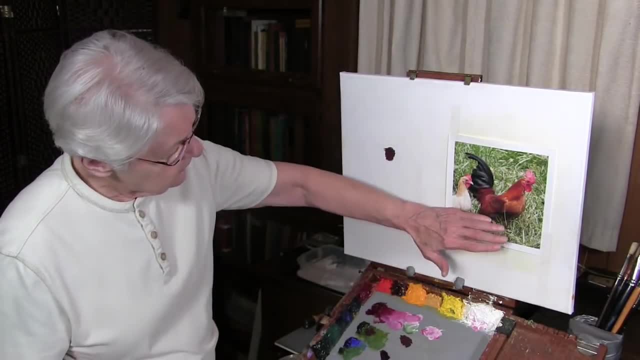 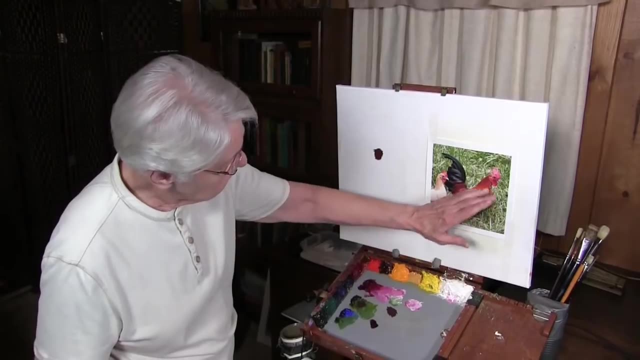 looking at the color, You're looking at value. So if I'm saying, all right, that's the darkest value, What is the lightest value I'm looking at? Now, if I'm looking at the whole rooster, probably if I squint and squint, close one eye and squint the other one. 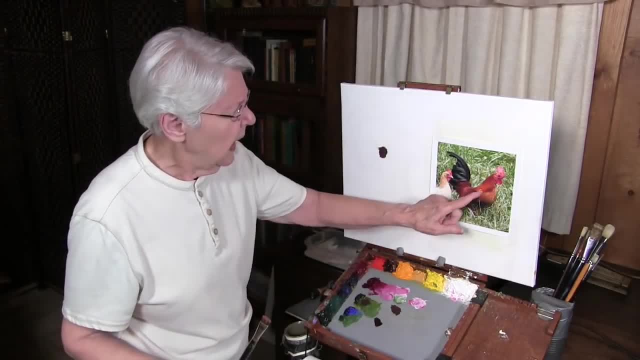 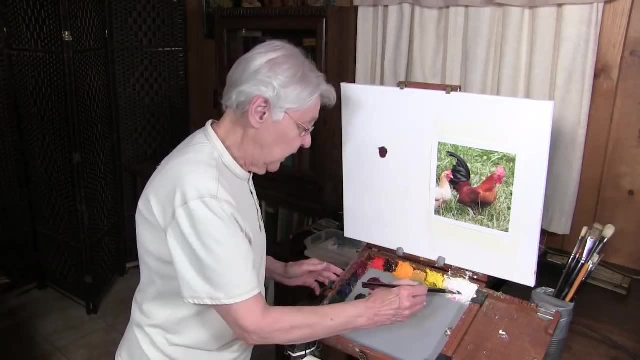 that helps to block details out so you can see value better. I see right here as being the lightest value of that, So that appears to be in the red. Let's find out. So if I can mix a little bit of a red, 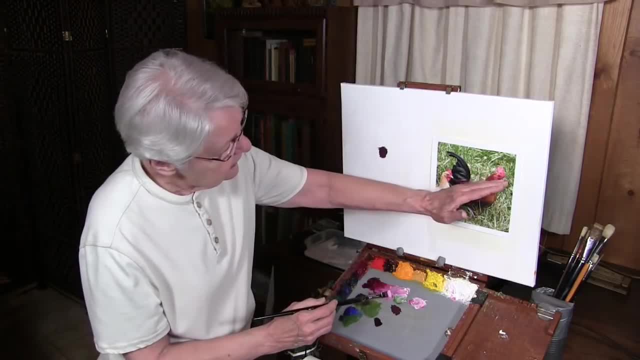 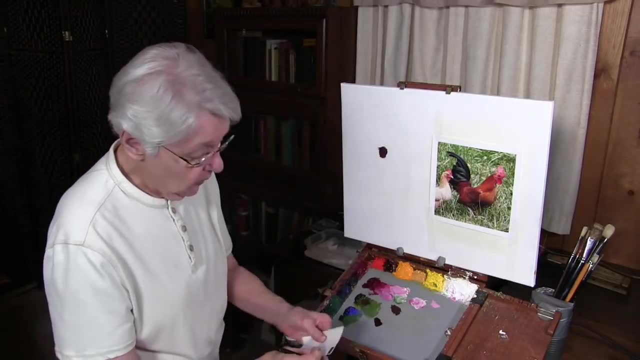 And a light value. and it is in. it is not in shadow, It has light shining on it. So if I can mix a little bit of that and right on my same piece of paper here, right on the edge, I can compare those two and say, no, I'm a little dark. 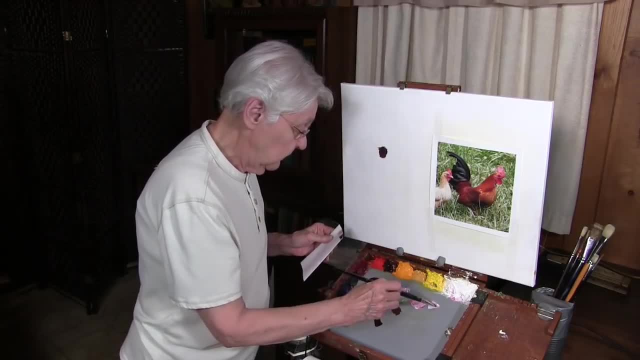 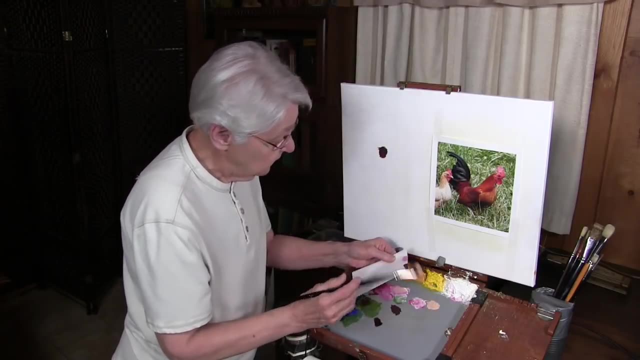 That means I need to add light. Now I can add a little bit of yellow to that. Now let's see, Do I have it, Do I have that value yet? So now I can go on the other side. I can go on the other side of the piece of paper and squint and say, no, I made it too light. 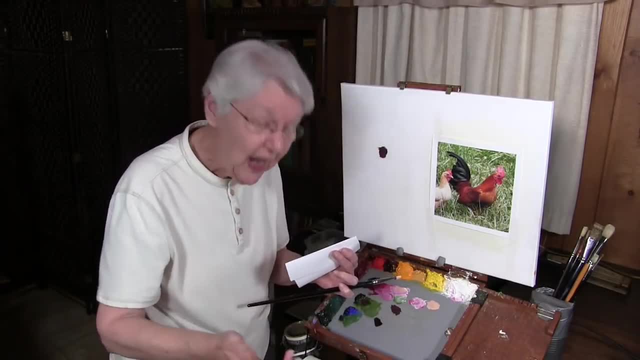 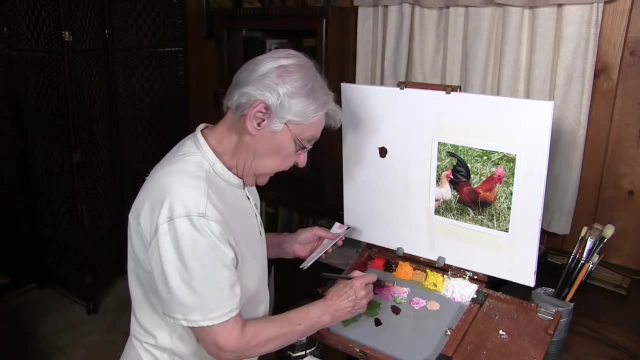 You see, you don't have to, you don't have to get uptight about it, You just experiment, Experiment by trial and error, And so I can add a little bit. Now let's see how much too light It's. um, yeah, 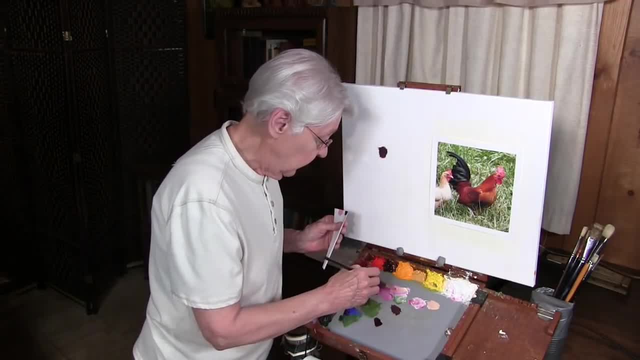 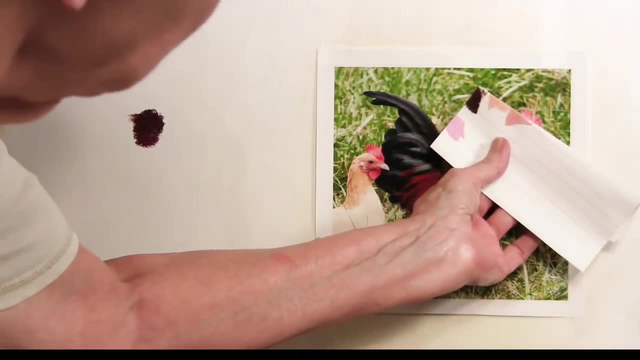 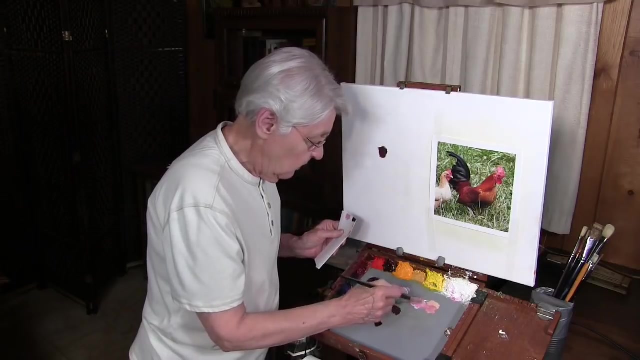 Needs to add another, another little bit of that, That red, to that, Make it a little bit darker. Now I can put this same place and hold that up. I'm getting closer, getting closer, so so I adjust it if it feels, if it needs to. 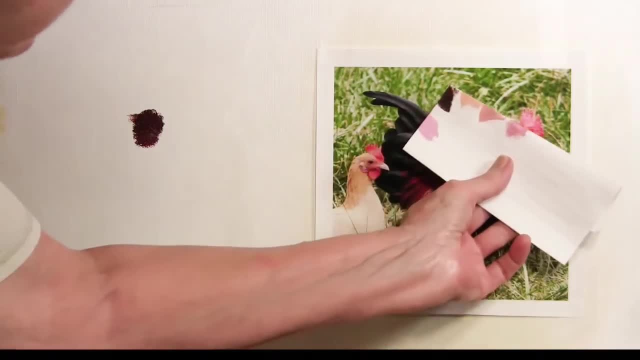 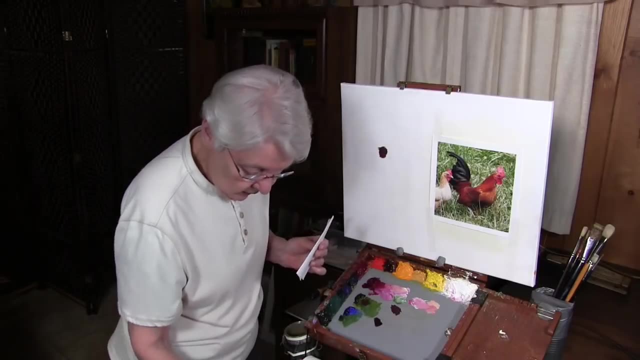 be lighter, I make it lighter. if it needs to be a little redder, I make it a little redder. now let's see what we have now. if you squint you see it's pretty much in the same value area. now, one thing I can do at this point is to compare those two. 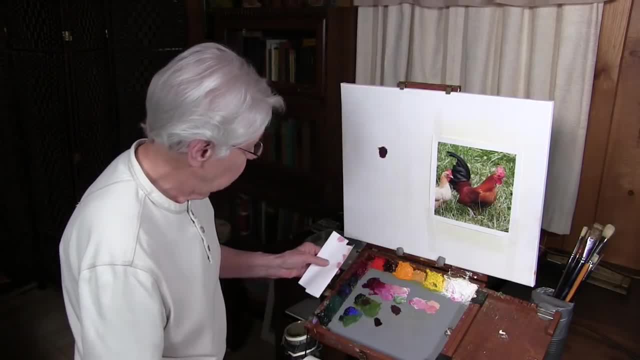 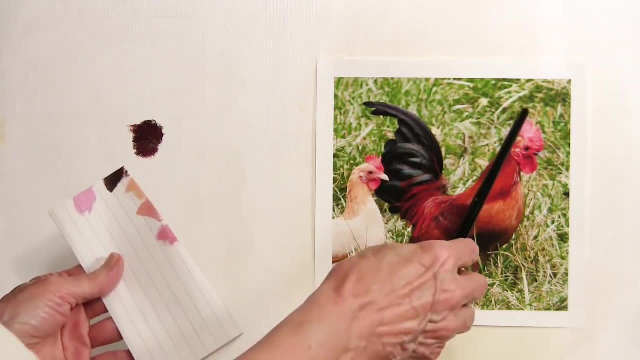 together the lightest light with the darkest dark. so I'm holding this up here. I see this is very light, this is very dark, this is very light. so I know then, if that's the lightest light I'm looking at and this is the dark is dark then 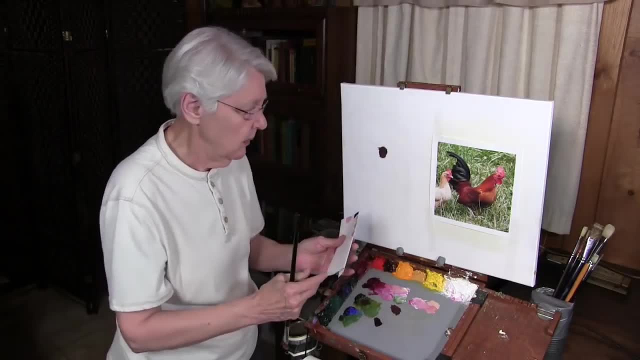 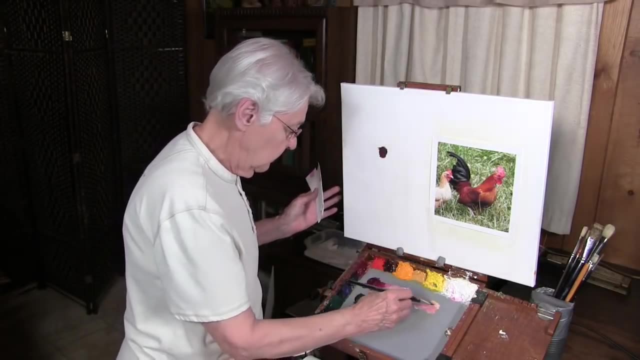 these are going to be somewhere in between that in value, so let's, let's look at that just a little bit longer. this is the darkest dark right here. well, I was gonna- I won't make this light the lightest light there- to the na kommen layer. 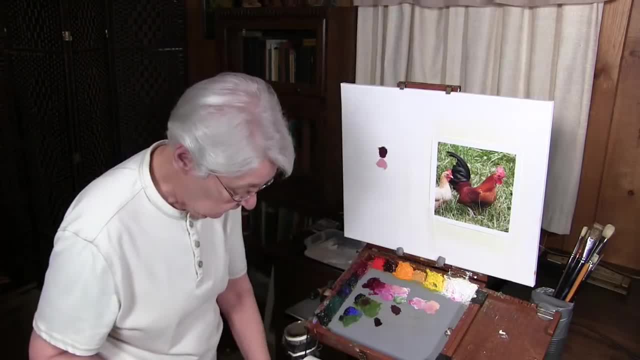 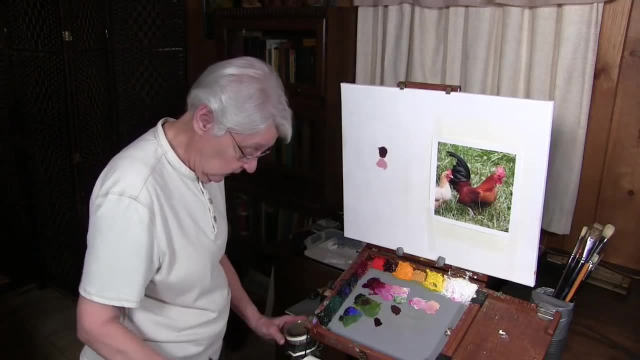 light. right there Now we have the darkest dark and the lightest light. It will be a lot easier to look at the other values of the other colors in comparison. So if we think of in shadow, not in shadow, What's in shadow, What's? 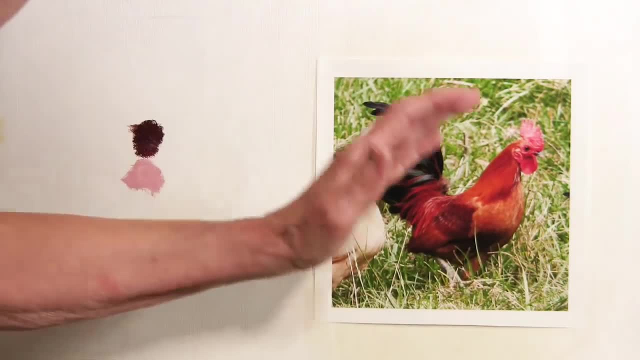 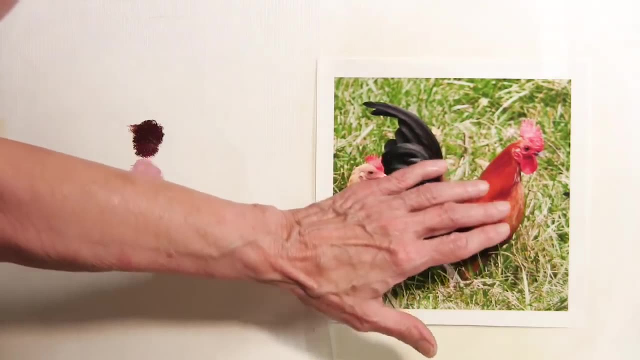 not in shadow. There's not really a bright light shining on that, It's kind of a subdued light. but we can see that this area right in here seems to be kind of in between light and shadow, So we can look at this area right here. 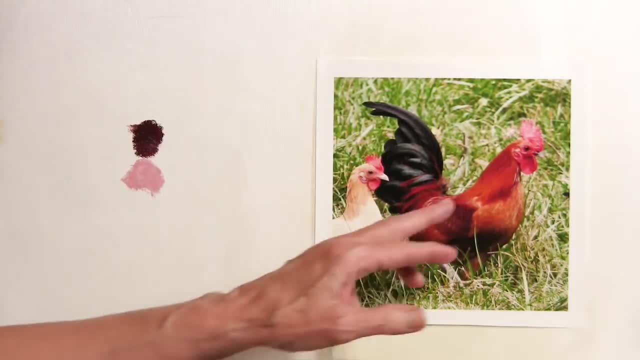 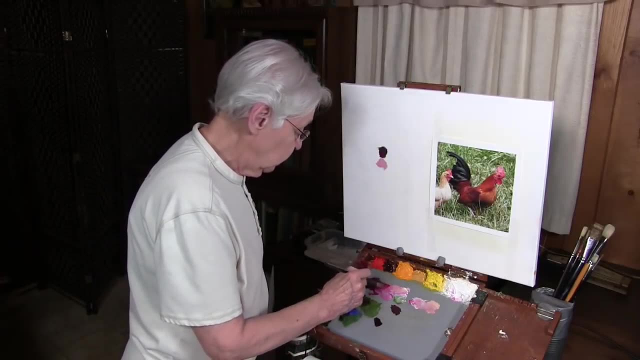 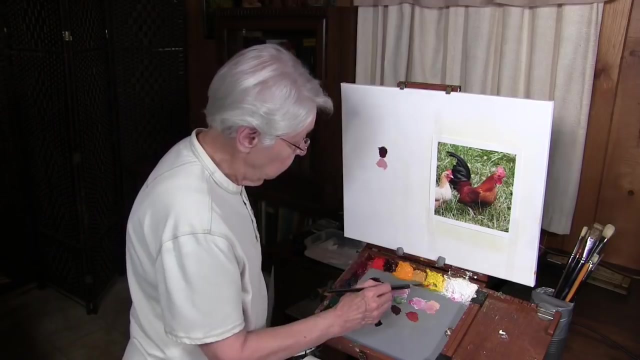 What value is that? All right, we know it's not this dark, We know it's not this light, so what we can reach for is something in between, And so then I might go into a red here, I might add a yellow to the red, and I'm looking for a value. 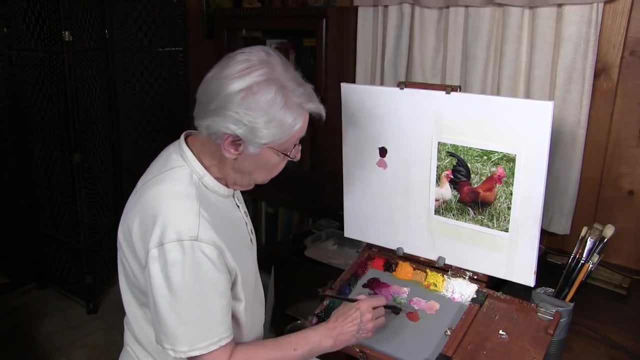 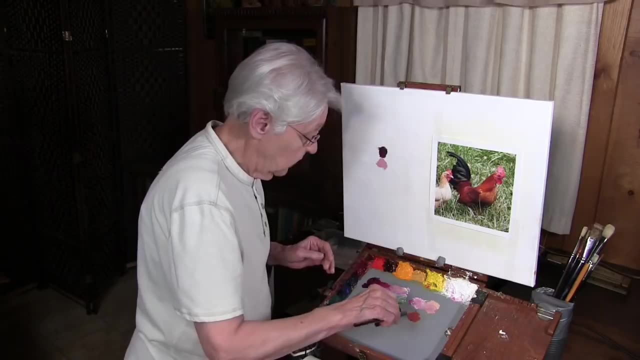 that is in between. And another way to do that is simply, if you're thinking of a black and white色 and you're starting to think of If you're working from a photograph, it's simply to hold your brush up next to it. 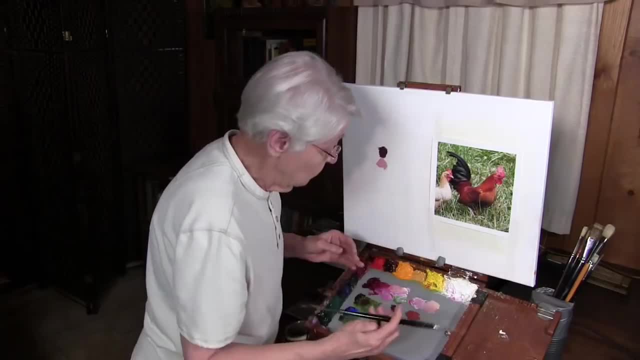 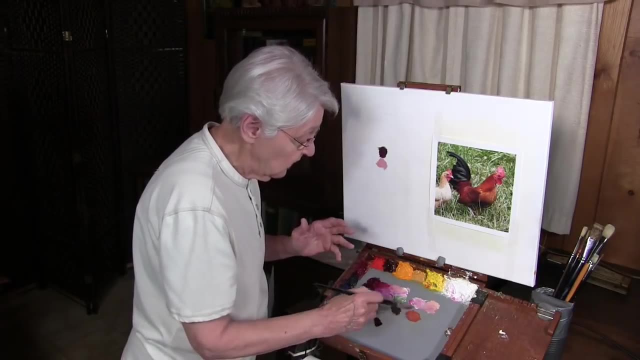 Now you see, when I squint I can see that that mixture I have on the brush is a little bit too dark. So that's the way you compare it, That's the way you read. values is comparative. Is it too dark? Is it too light? 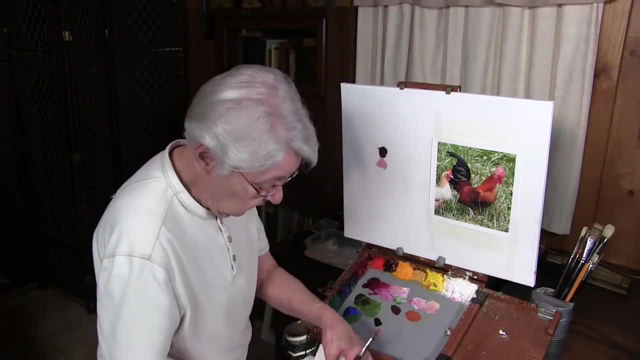 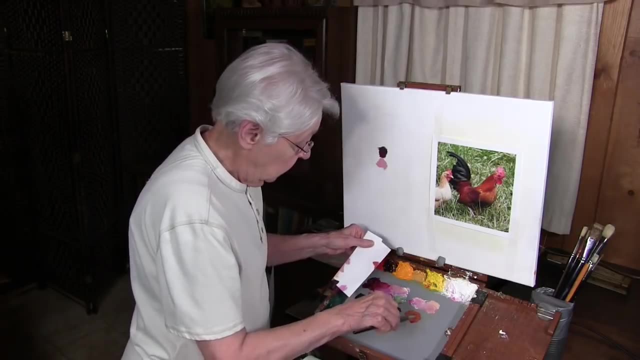 Now let's see. That's just about right. I can then do a real comparison. It needs to be a little bit more yellow. I think Not that that matters a whole lot, But you can also do the hue that way, by saying it doesn't need to be more yellow. 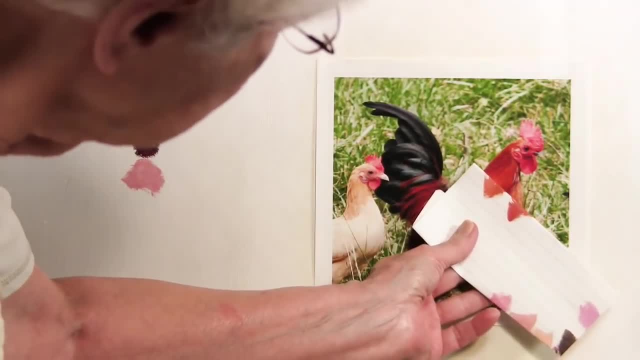 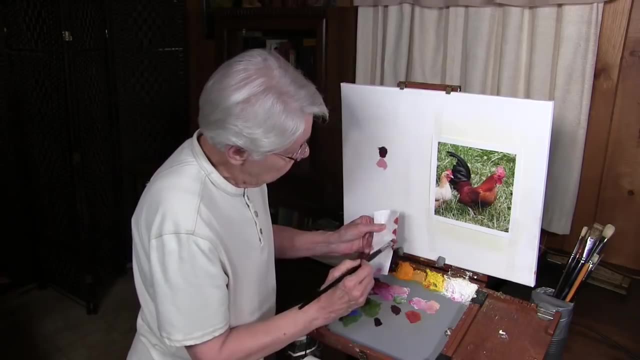 It doesn't need to be more red, But we're talking about values. Now we can see that is a bit too light. If it's a bit too light, I add the dark back to it. Now, let's try that. 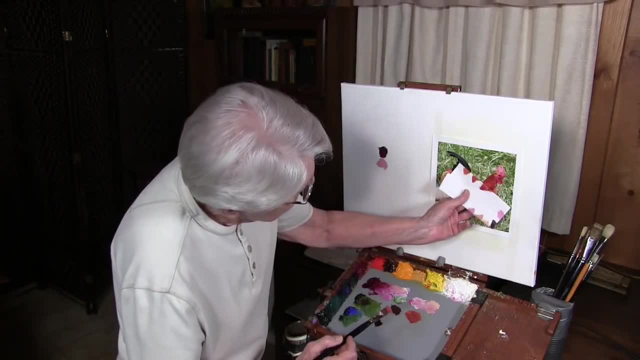 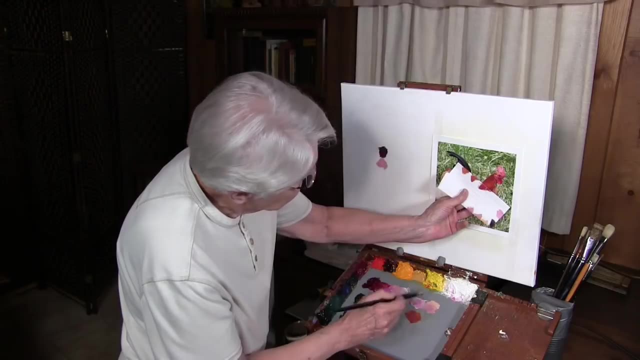 Right on the edge And that alright, I made it a little too dark. That means I add just a little bit more of the yellow and pull it back, A little bit more of the lighter color and pull it back, And there we have it, right there. 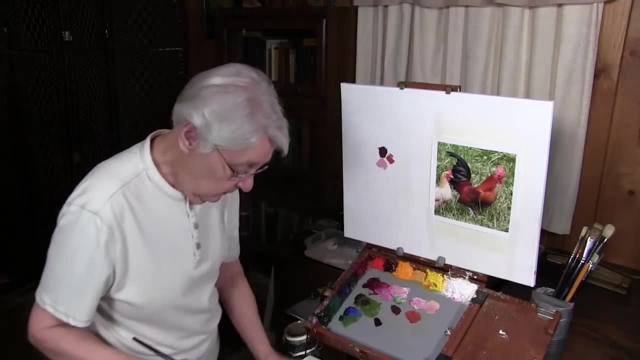 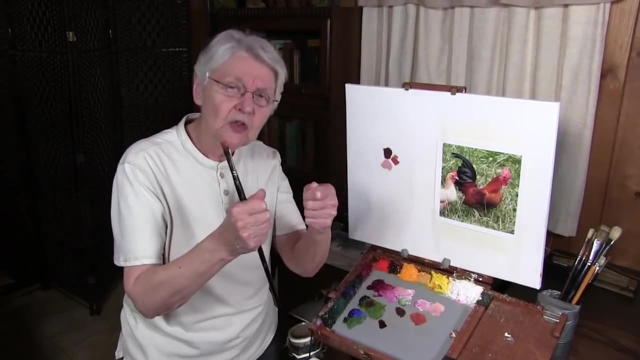 And this is the value we're looking at. So that is that will teach you to use that method of comparison: Comparing one value to another, Not just trying to hit a single value that you're looking at, But compare one value to another. 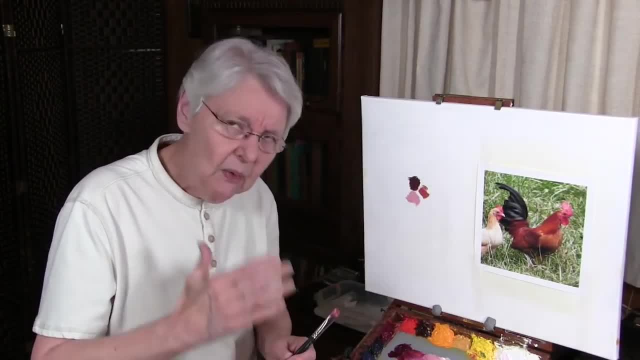 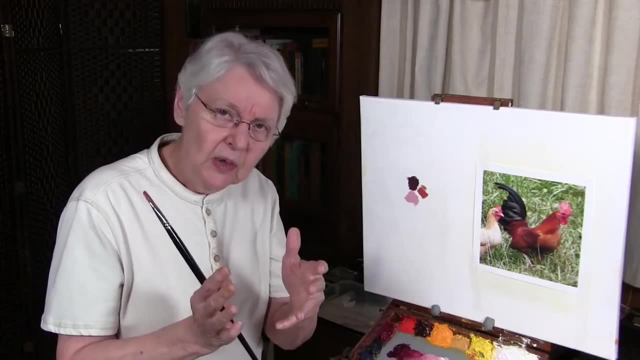 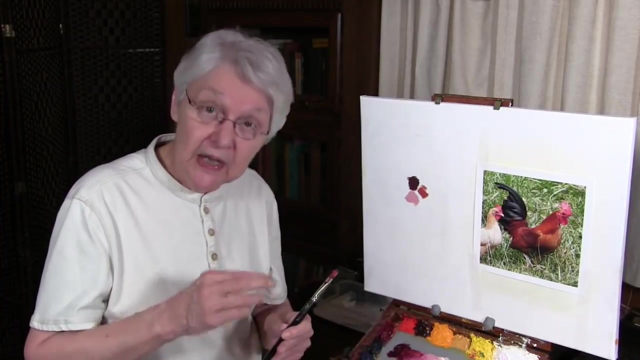 And be willing to work, play with the play, with this process of mixing and trying to match values The way you solve problems, The way you saw me doing it here. The more experience you have in in the actual mixing and matching of values, the easier it becomes. 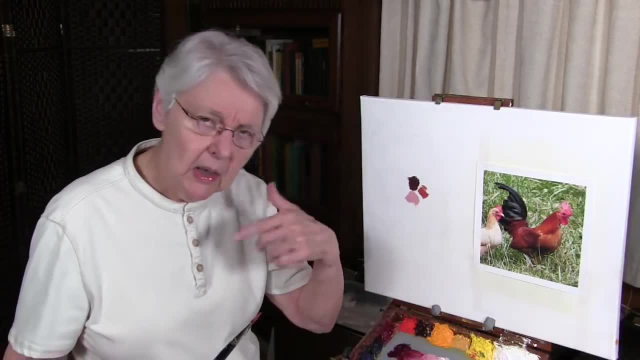 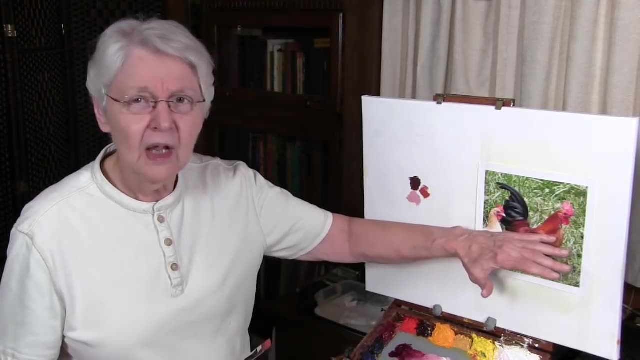 And the easier it becomes to see when you're looking at a value, to see exactly what value you're looking at. So I suggest that you get to work and do lots and lots and lots of value comparison, Mixing paint and matching values that you see.